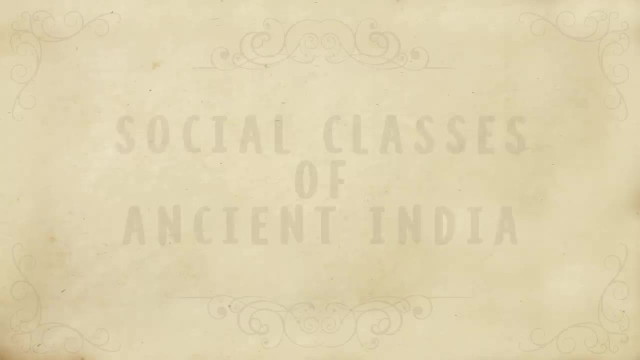 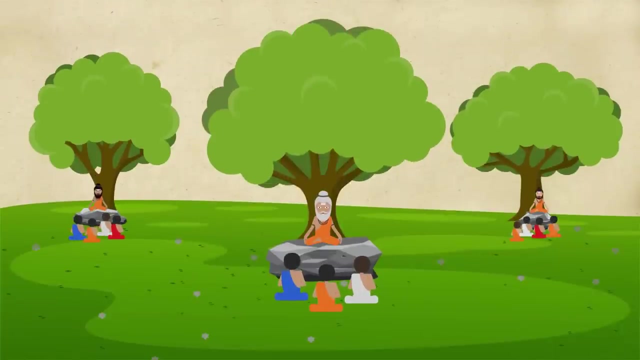 This video will detail in what ways the ancient Indians were divided into social classes and in what ways social classes of ancient India reflected the attitudes, beliefs and needs of ancient Indian society. The term social classes through a historian's lens means how a civilization is divided into classes that have different roles, responsibilities. 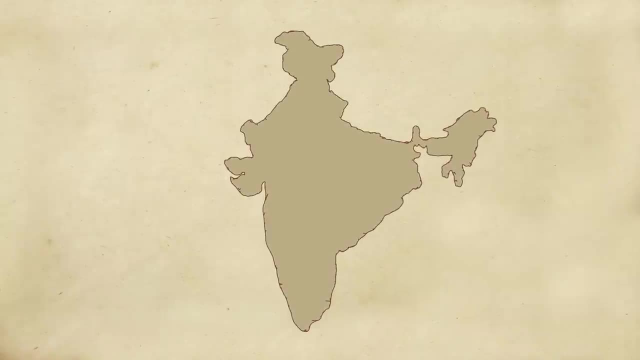 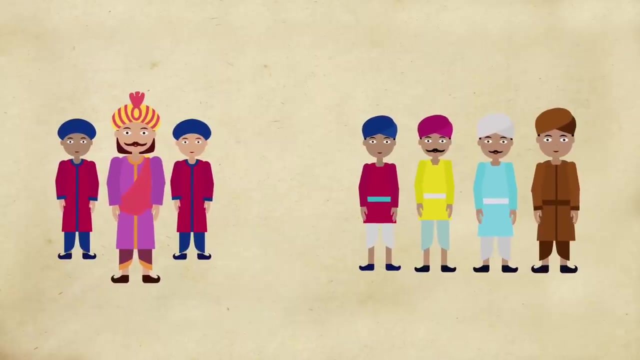 and privileges. For example, most ancient civilizations are ruled by kings and governed locally by nobles. A working class of farmers and laborers made up most of the population and in some cases, the lowest class were slaves. How were the people of ancient India? 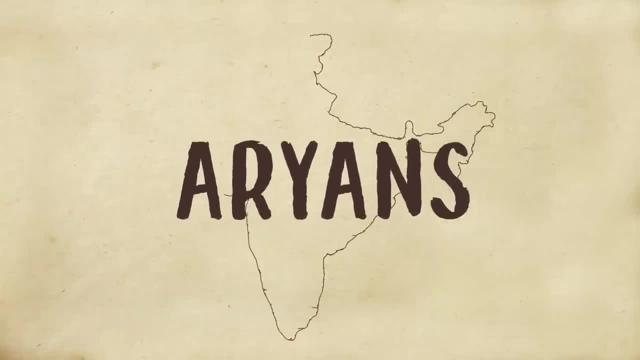 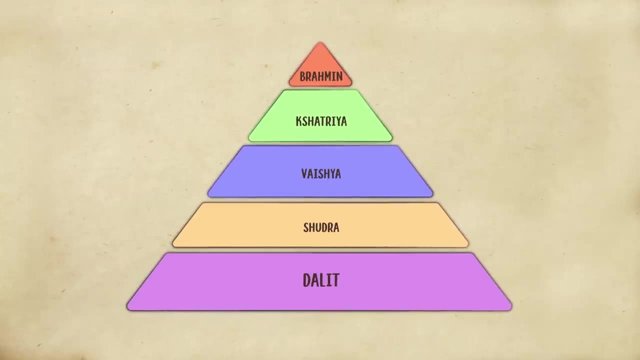 divided into social classes. The Aryans brought the caste system to ancient India, creating a strict social ladder. Each group was a different varna or social class in ancient India. Let's take a closer look at each varna, in order from the most to the least significant in India's society. 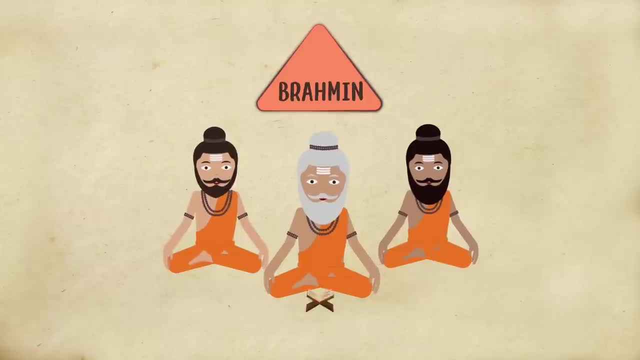 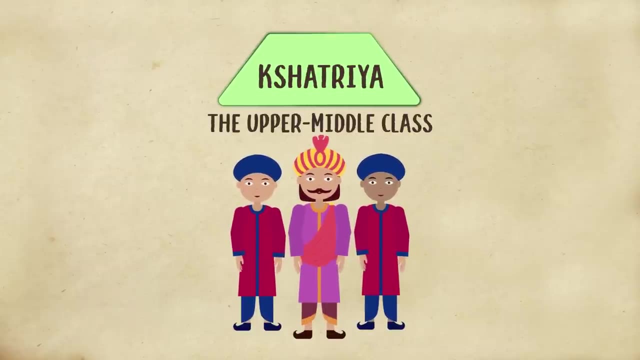 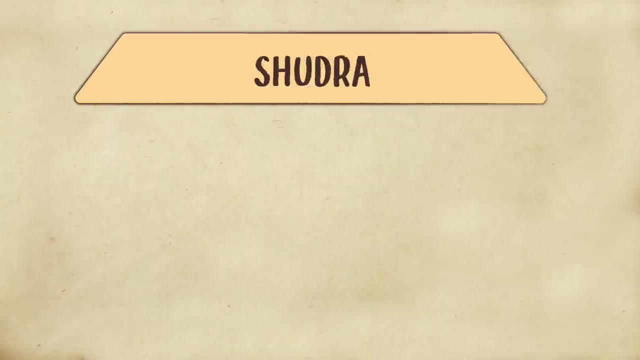 The Brahmins, or top social class, were priests, scholars and later Hindu gurus or teachers. Next were the Kshatriyas, or the upper middle class, who were kings and warriors. The Vaishyas, or the middle class, made up businessmen, traders and farm owners. The Shudras were 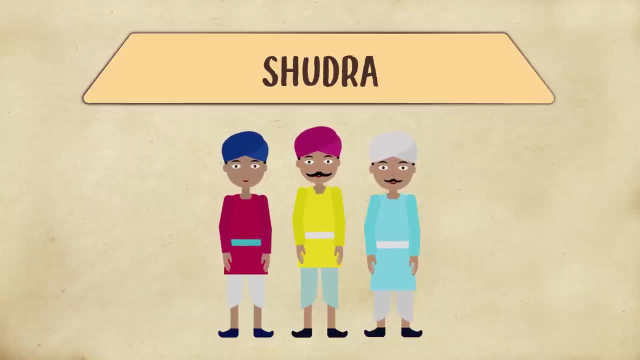 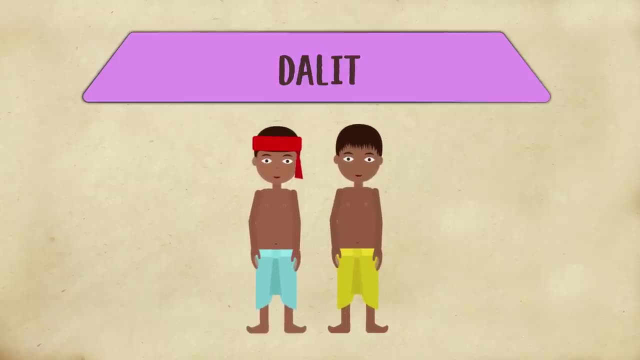 servants or unskilled farmers, considered inferior to the other castes mentioned above. Lastly, at the bottom… were the Dalit, or untouchables, who were laborers that did the lowest and worst of jobs. though they were not slaves, They were considered unclean and were often forced to. 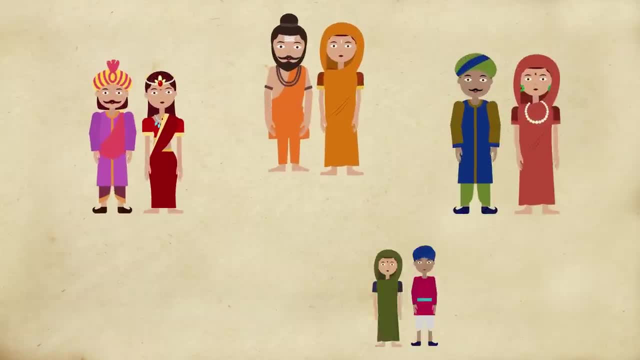 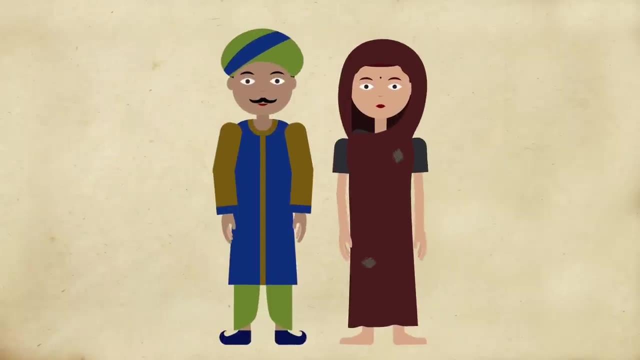 live outside of villages. While it's unfair, once a person is born into one of five groups, they have little to no chance of moving into different varnas. People were prohibited to marry outside of their own varna. They lived in communities with each other and were often 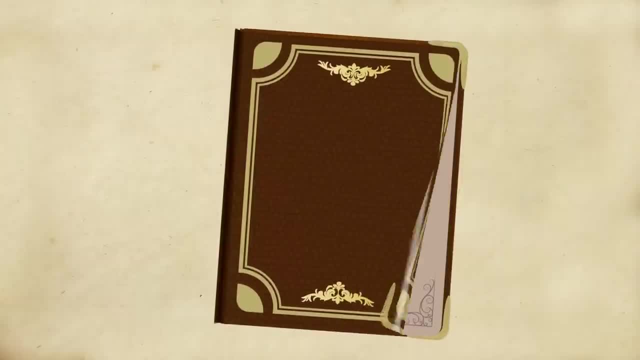 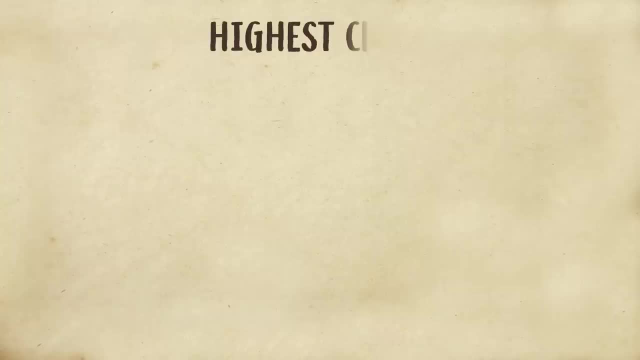 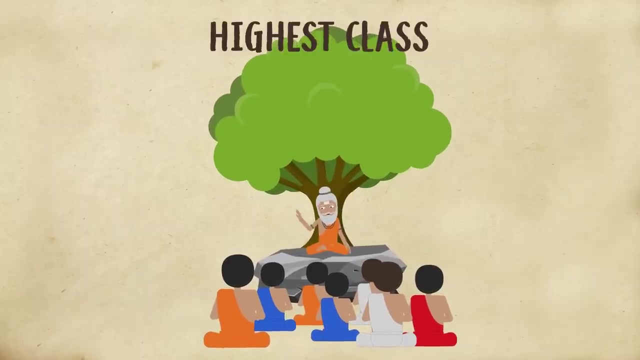 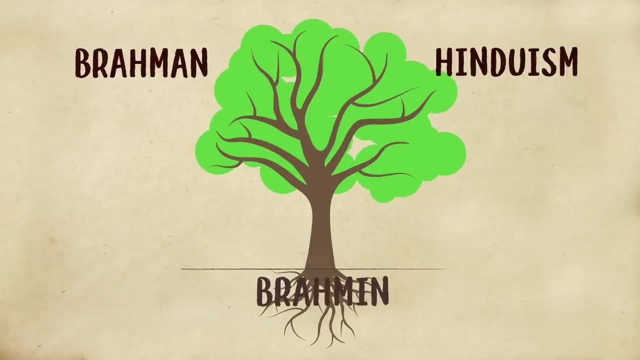 forbidden to mingle with other varnas. In what ways did social classes of ancient India- the lowest class intersect and the lowest class associate with each other? reflect the attitudes, beliefs and needs of ancient India society? The highest social class, the Brahmins, were those directly connected.